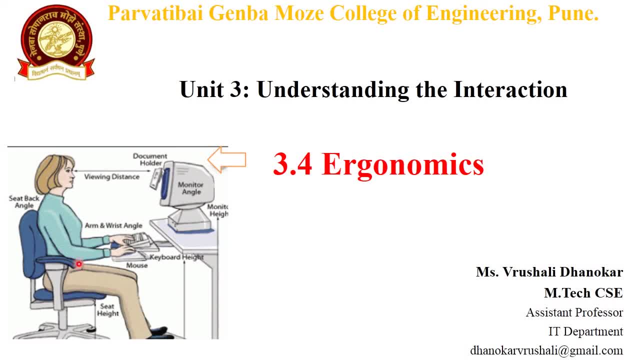 Good morning everyone. I am Rishali Dhanokar, Assistant Professor, IT Department. In my last video, we learned about Donald Norman's model. Now in this video, we will learn about ergonomics concept. Okay, So let's see what is mean by ergonomics. But before start the session now see here this diagram: show the exact concept of ergonomics: Proper viewing distance. 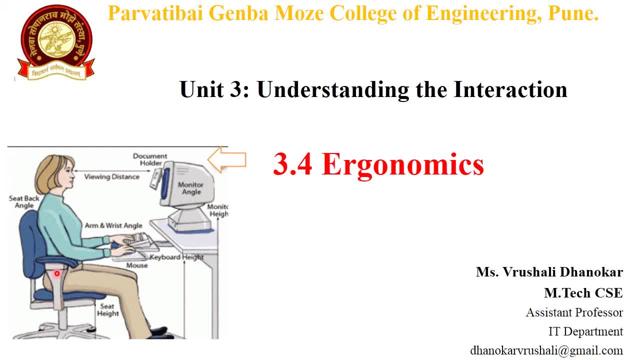 between the human and the system: the proper sit back angle, armrest angle, then monitor angle, etc. Also proper height, keyboard height, mouse height, then monitor height, etc. So this is the concept of ergonomics. So let's see definition of ergonomics Next. 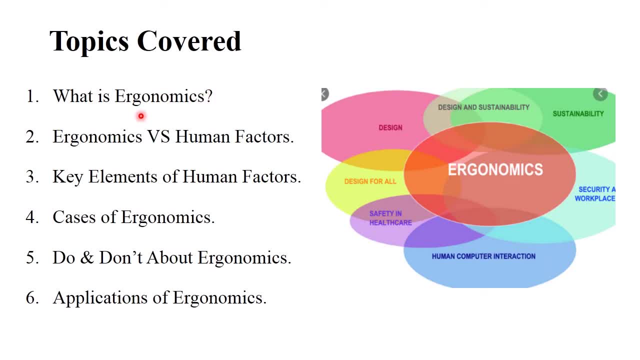 Following points are covered in this video, which includes: what is ergonomics, ergonomics and human factors, Key elements of human factors, cases of ergonomics, and there are some do and don'ts about ergonomics and application of ergonomics. Next, 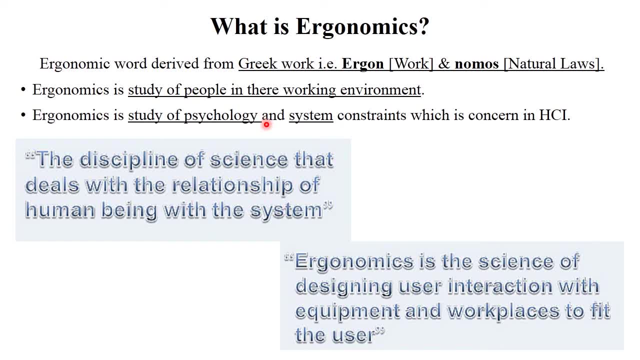 So what is mean by ergonomics? Actually, ergonomics is a Greek word where ergon means work and norms means natural laws Means by using natural laws, you have to do particular work. This is the concept of ergonomics. 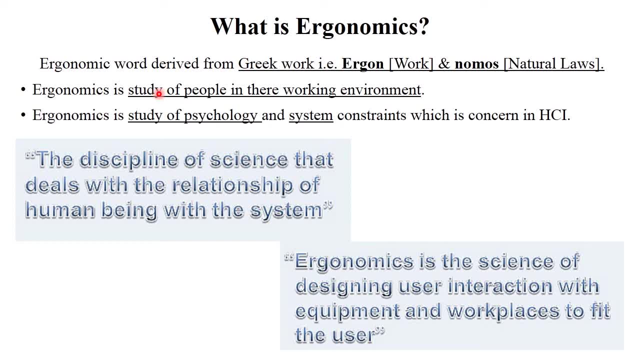 Again, there are many reasons for ergonomics. Once again, there are many definitions or many terms about ergonomics, but meaning is same. Ergonomics is a study of people in the working environment, How people are work in their working environment. Ergonomics is a study of psychology and system constraint, which is concern in HCI. There are also some definitions of ergonomics, like the discipline of science that deals with the relationship of human being with the system, How exactly human is, handle each and every part of the human being's life. There are 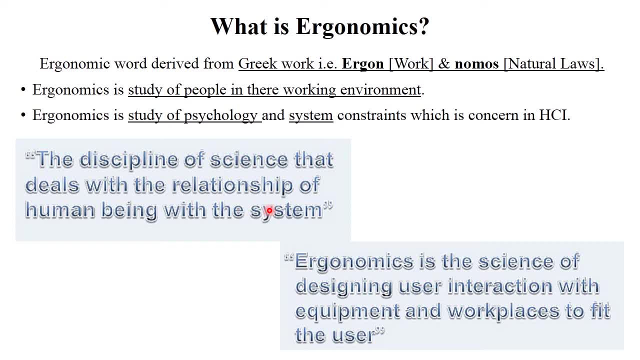 of the system, like keyboard mouse, monitor, etc. the study of those which is called as ergonomics. ergonomics is a science of designing user interaction with the equipment and workplace to fit the user each and every part of the system. keyboard mouse: it's very easy to use in proper manner. the study of this. 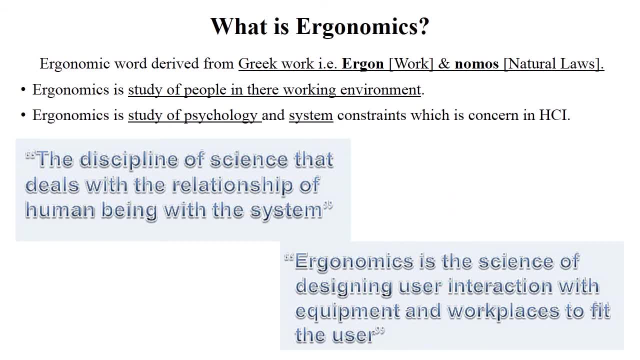 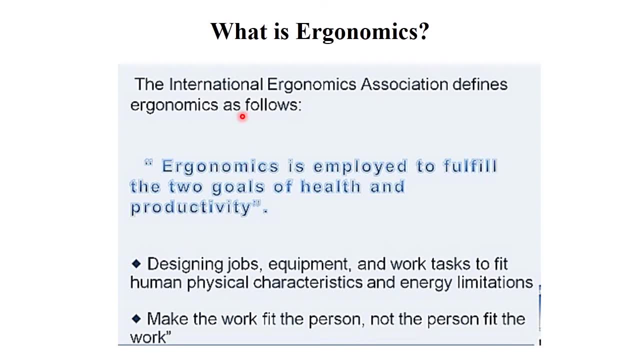 all things which is called as ergonomics. clear. next, now again, the international economics Association defines the ergonomics as follow: ergonomics is a employed to fulfill the two goals of health and productivity by using proper parts of the system. you have to improve your health and the productivity. this is 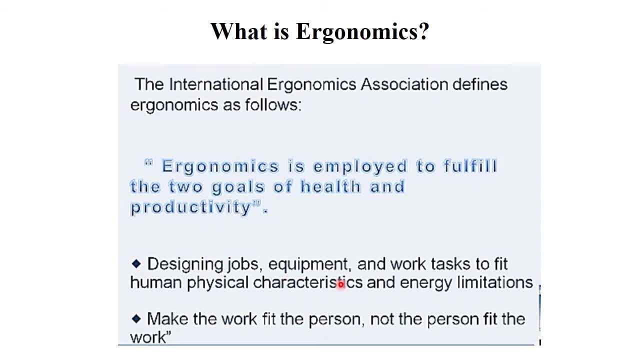 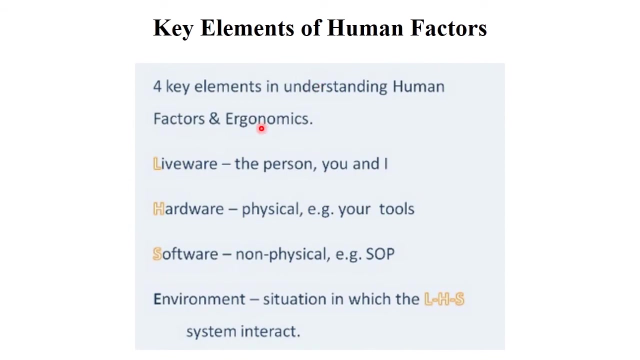 called as economics, to designing job equipment and work tasks to fit the human physical characteristics and energy limitation. so ergonomic simply means make the work fit the person, not the person fit the work clear. so let's see in detail how exactly economics are work next. okay, before that, there are key elements of human factor, 4 key elements in: 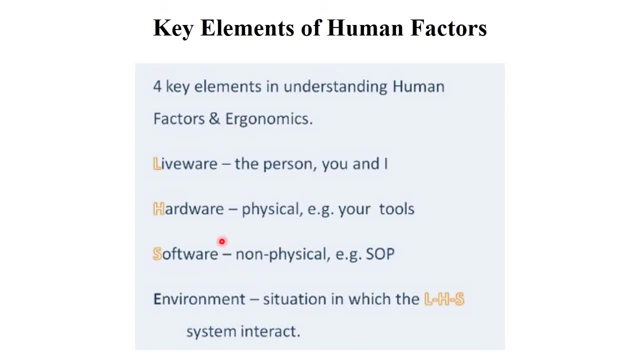 understanding human factors and ergonomics. see here. ergonomic is a study of software- ROSTIE & HANNAND pelo Class hardware and liveware. software includes all the non-physical characteristics, means operating systems, etc. and hardware includes each and every tool which is physical, means you have to touch each and everything. this is called as. 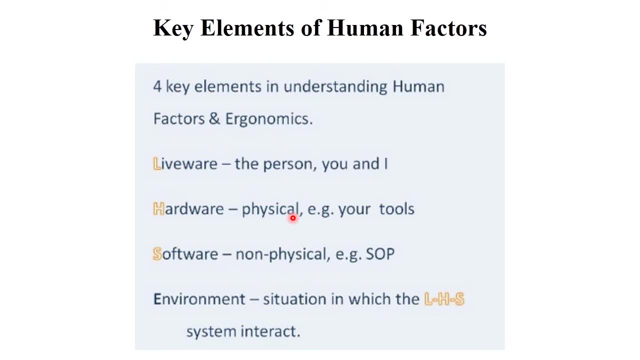 hardware part like keyboard, mouse, monitor, CPU, etc. right so the interaction between human with this software and hardware term, this is called as live fair. life fair means the person, you and I- right the environment where all the life fair, hardware and software, this interaction is work. these are the key. 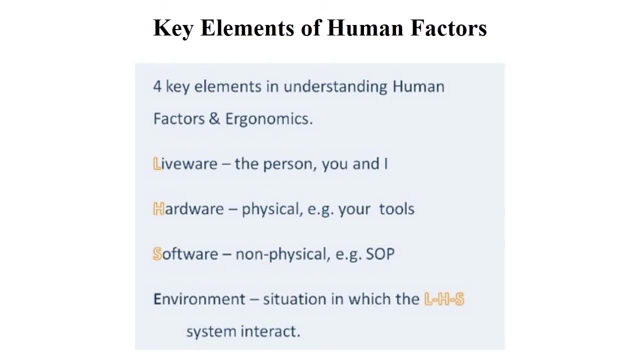 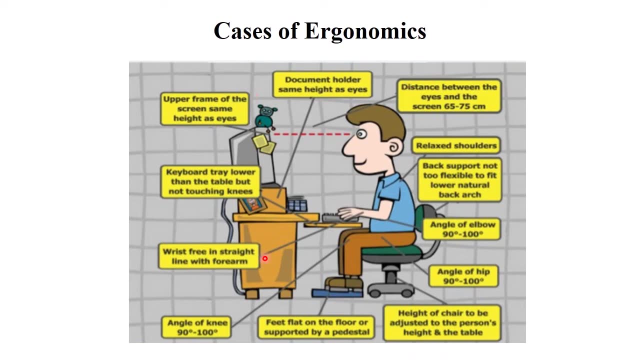 factors of ergonomics clear. next now see here the cases of ergonomics. this is complete structure of ergonomics. ergonomics means to study of distance between the eye and the screen. there is minimum 65 to 75 centimeter distance is necessary. 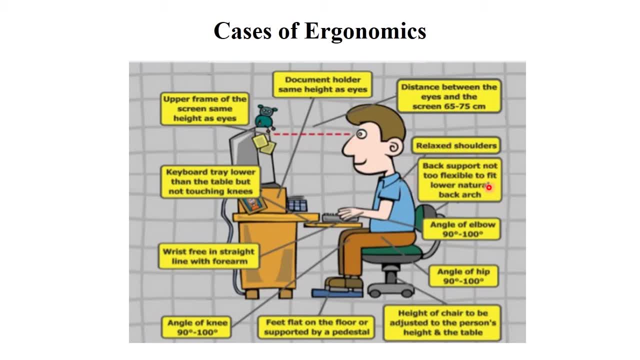 also there is relax shoulder back support, not too flexible to fit the lower natural back arc right and the angle between. but while using keyboard and mouse, the angle between your hand with 90 degree of 200 degree. the angle of hip is 90 degree, 200 degree. the proper sitting arrangement is necessary. 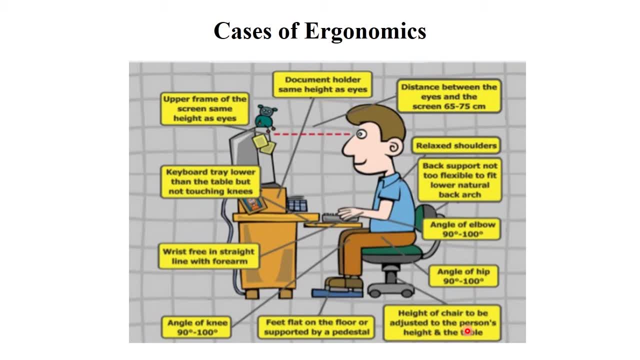 then height of chair be adjusted to the person's height and the table. that's why there are many industries and organization wheelchairs are used, fit flat on the floor and supported by the pedestal. clear the angle of knee. angle of knee is always between 90 degree to 100 degree. wrist free. 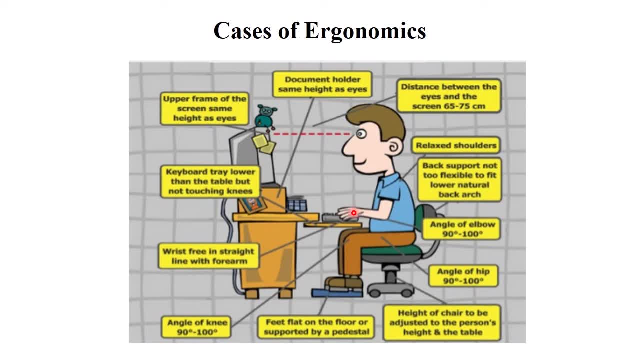 is strength line with the forearm properly. you have to use your keyboard in proper angle keyboard tray lower than the table but not too touching needs. this is your monitor. after that there is keyboard and mouse. the place of keyboard and mouse always lower than monitor, so it's easy to use. then upper frame of the screen, same height of the eye. the screen of 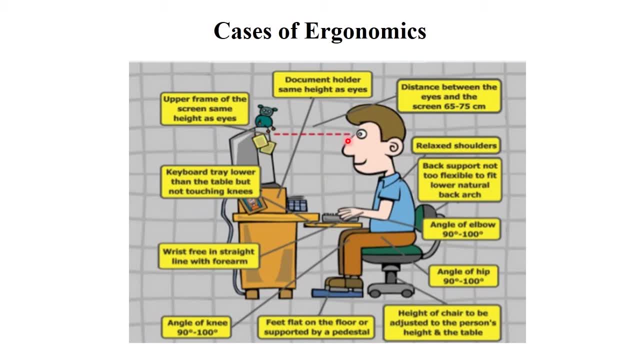 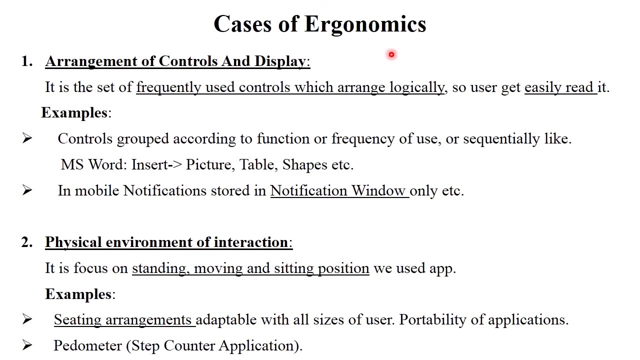 the monitor and the eye. it is in same manner, so documents holder same height as eyes. clear. so study of all those things which is called as ergonomics, clear. next now there are four cases of ergonomics. ergonomics always work in four cases. let's: 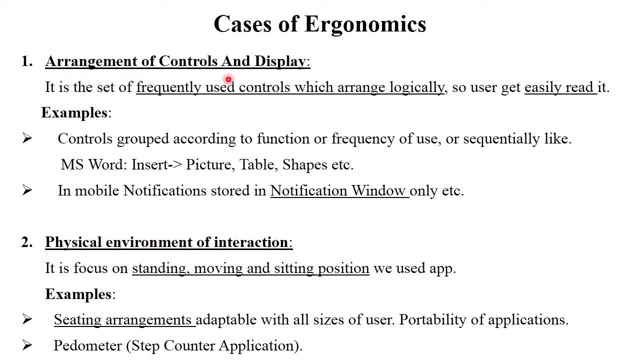 see first case. the first is arrangement of controls and display. it is a set of frequently used control which arrange logically and properly so users get easily read it, for example, while using Microsoft word: okay, there is insert, menu bar is given. okay, in insert there is picture table shapes. all these options are included. 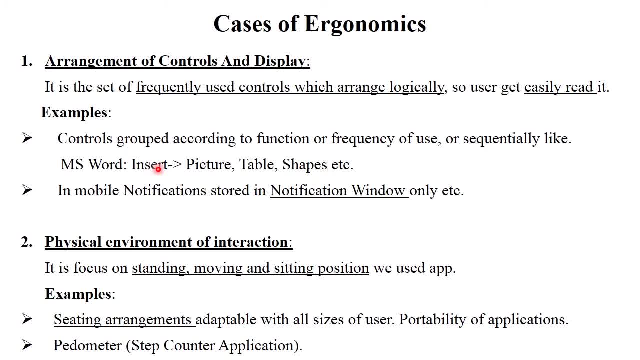 or combined. right again, there is file option, then edit option. in edit there is cut copy paste. these options are combined with each other. so this is called as proper arrangement. logically they are easily arranged with each other. clear. so control group according the function, the frequency of use or sequentially. 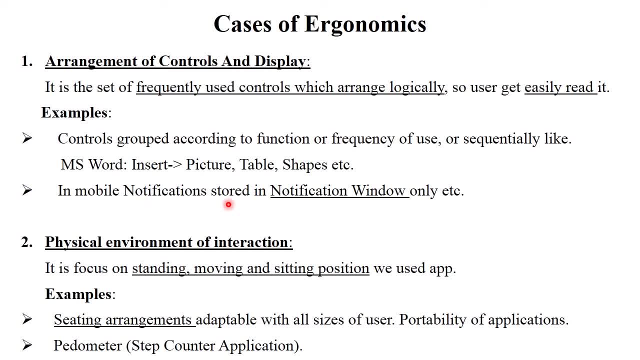 again. the another example is mobile notification. all the notifications are stored into the notification window only. so this is the concept of ergonomics: so users get easily read it or easily access it clear. the next case is physical environment of interaction. it is focus on standing, moving and sitting position while using the application. okay, the examples. 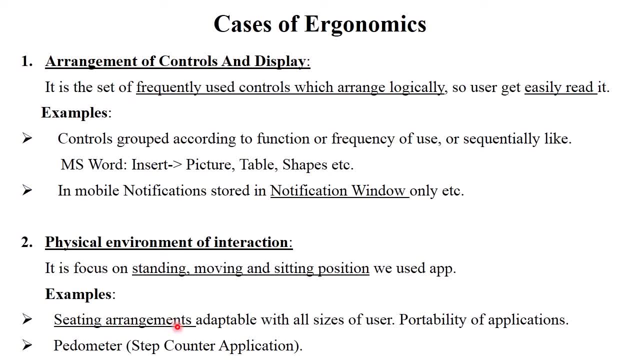 are sitting arrangements adaptable with all size of the app, eg a book with a date of date你用下 sit in. there's another case of moving printed paper sitting against a wall and bearing of Ciagro's Saskatchewan technology. the seconday case is mobile teampt uncle Data tone device 딀. 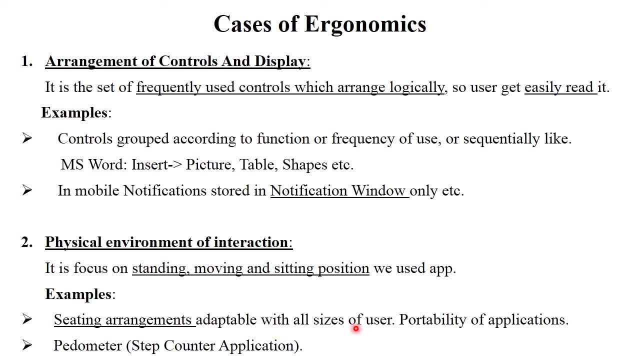 the user: mobile, tap, laptop. these are all the portable applications. portable means moving applications, right, but computer or desktop is not the moving application. so according to this ergonomics, laptop, tap, mobile- it's very easy to use because they are portable. again, another example is pedometer. pedometer is a step counter application. while walking, they count the steps of each and 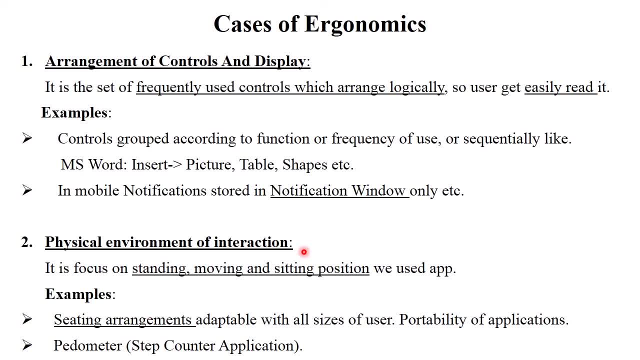 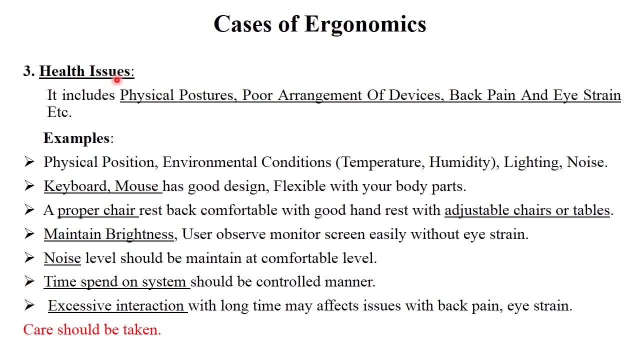 every person right. so this is the concept of ergonomics. next, okay, the next main case of ergonomics is health issues. ergonomics mostly focus on the health issues. it includes physical postures, poor arrangement of devices, back pain, eye strain, etc. so let's see the examples of health issues. see here physical position, environment conditions. 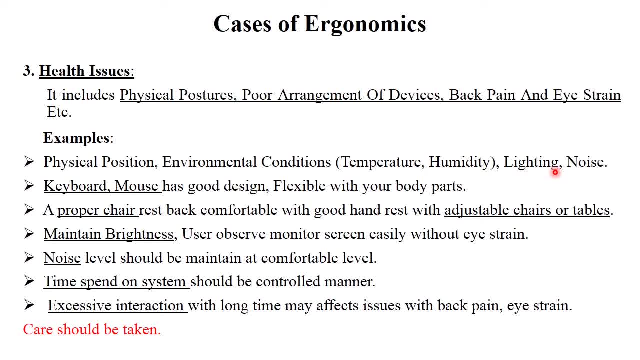 which includes temperature, humidity, lightning, noise. this also affects on the system as well as human. keyboard and mouse has a good design, flexible with your body parts. right. you have to easily use keyboard and mouse in proper manner, in proper angle, then proper chair. if you have lots of works on computer, so proper chair is a useful tool. so let's see the examples of health issues. 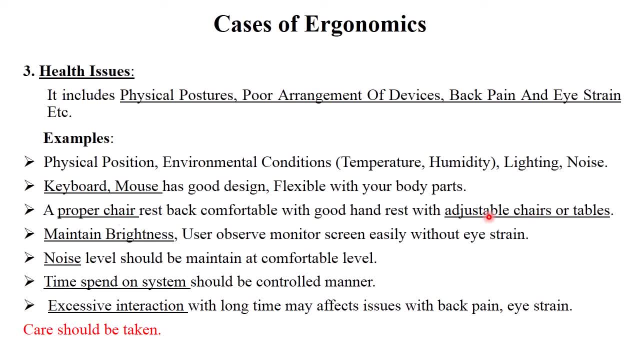 so here: physical position, environment conditions, which includes temperature, humidity, lightning, noise. So proper chair or adjustable chairs or tables are necessary because it rests back, comfortable with a good hand, rest Clear. Next again, maintaining brightness. User observe monitor screen easily without eye strain. So you have to maintain the brightness of your screen. 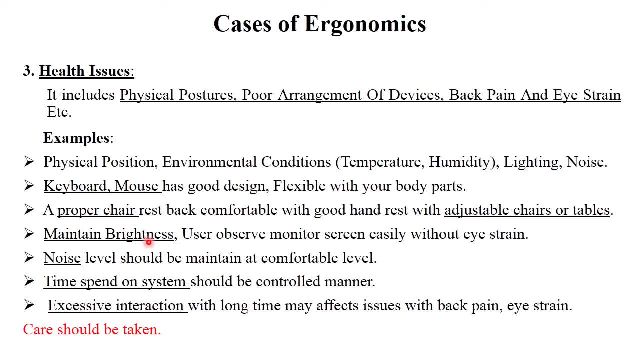 Laptop computers as well as mobile. you have to maintain the brightness Clear. The next one is noise level. Noise level should be maintained at comfortable level. Once spent on, system should be controlled manner. You have the proper control on yourself while using the systems, mobiles, laptops, etc. 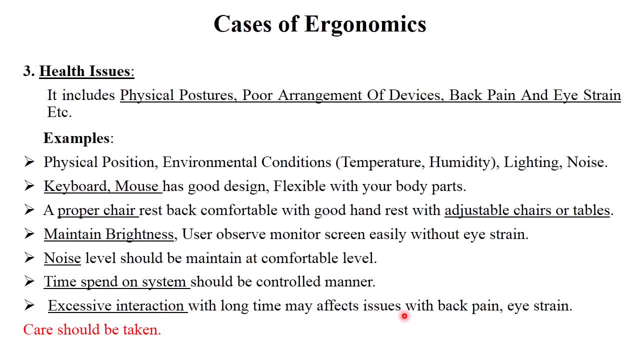 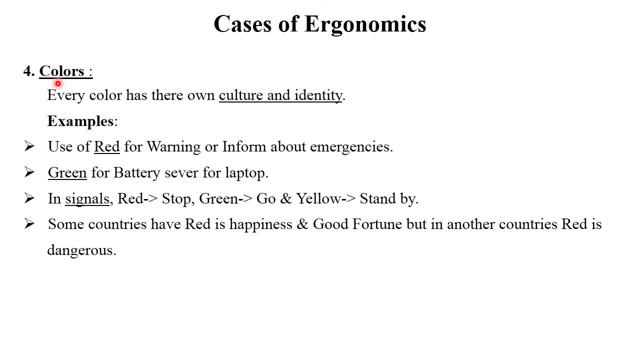 The excessive interaction with long time may affects your issue with back pain, eye strains, etc. So care should be taken. So, while studying all those things, this is called as ergonomics Clear. Next, The last case of ergonomics is color. Every color has their own culture. 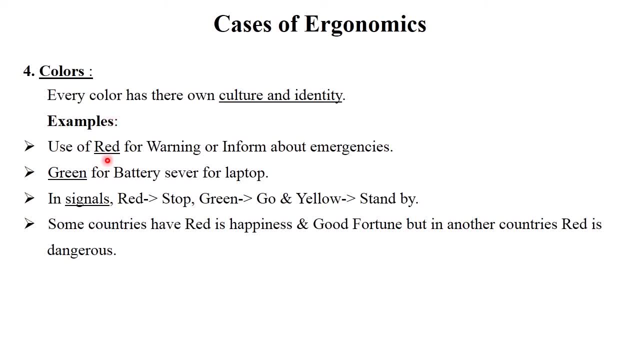 For example, use of red. Red indicates the warning or inform about emergencies. Green color indicate battery saver for laptop. So these are the identity According the color. you have to find out. the particular thing related to the color Again signals, that is, red means stop, green means go, yellow means standby, etc. 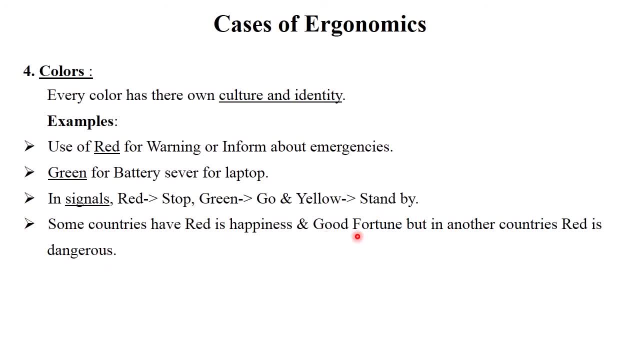 Some countries have red means happiness and good fortune, but in another countries red means dangerous. So it depends on culture, countries, identities and manner. So color is also affects on the human and tendency of human Clear. These are the all cases of ergonomics. 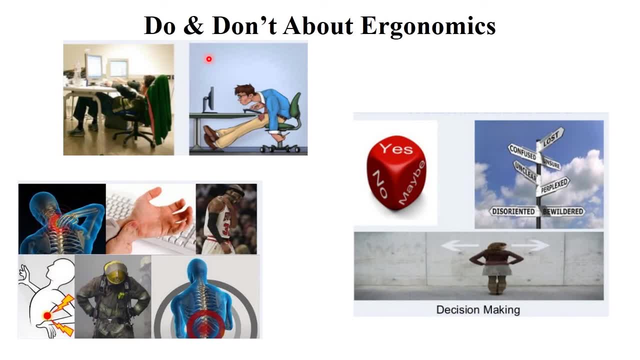 Ok, Next. Now there are some do and don'ts about ergonomics. The sitting position like this while using computer, which badly effect on muscles. pain, back pain- Again proper. If you not use properly keyboard and mouse it also. hand pain is also increases. 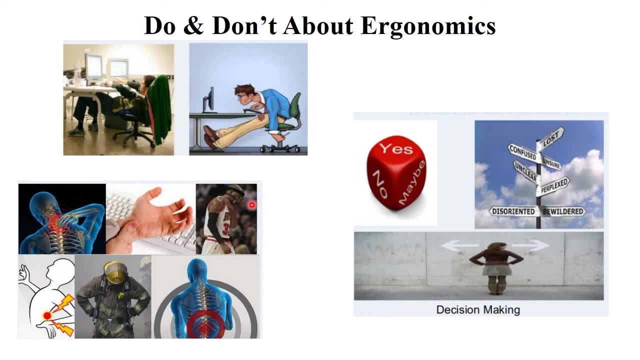 So you have to use proper thing or proper parts of the system in proper manner. Clear: If you have the proper decision making system, ok. If you move on, yes, no, maybe. so that's not possible. You have the proper decision making system. either yes or no. 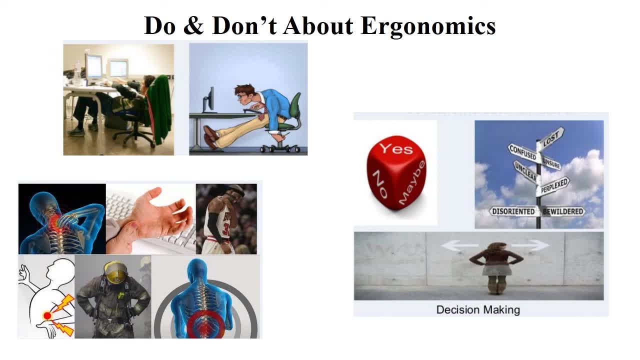 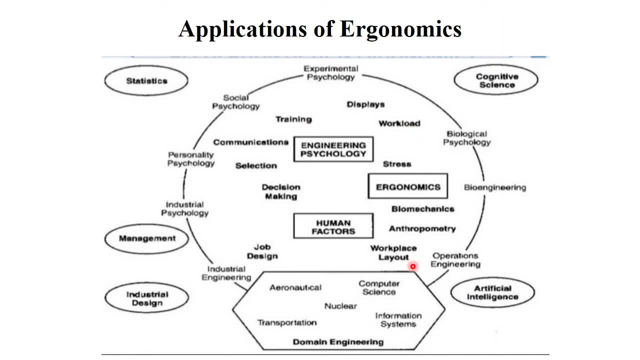 So this all affects on the ergonomics Clear. Next, Applications of ergonomics. I already explain in my previous video different multidisciplinary fields of human computer interaction right, So this all field where ergonomics concept is used, Like domain engineering, which includes aeronautical transportation, nuclear computer science. 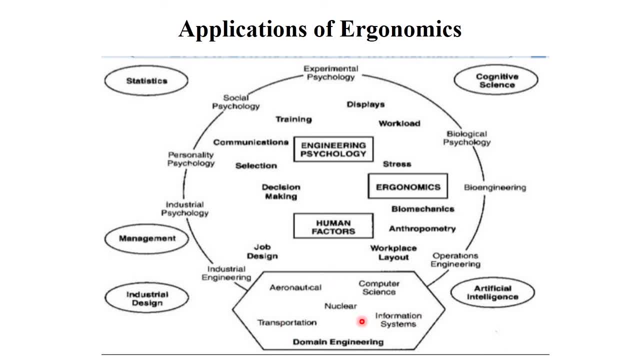 information system. In all fields computers are used. If you used computers in each and every field, Then you need to apply ergonomics concept. So you need to apply ergonomics cases. Then again, engineering, psychology, human factors like communication, decision making, job design. 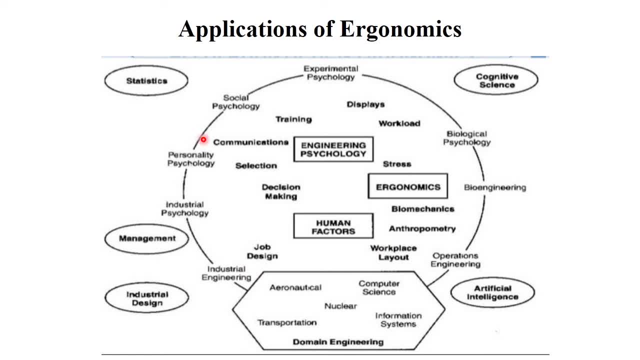 workplace layout. All these things are included in this field, Like industrial engineering, industrial psychology, personality psychology, social psychology, experimental psychology, biological psychology, bioengineering, operations. engineering means each and every field. computers are used Also: industrial design, management, statistics.